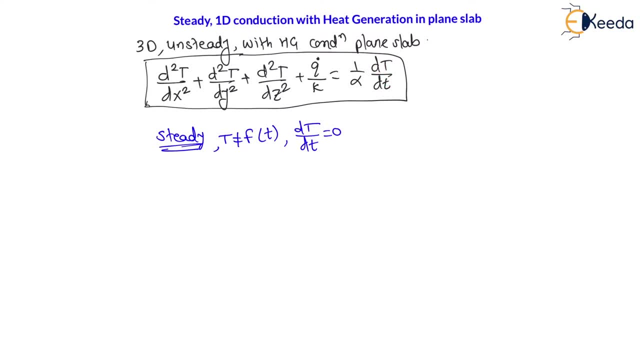 Here, capital T is for temperature, small t is for time. Alpha is thermal diffusivity and that we have learned. as alpha is equal to thermal conductivity divided by rho cp, Thermal conductivity divided by heat capacitor, This ratio is called thermal diffusivity. 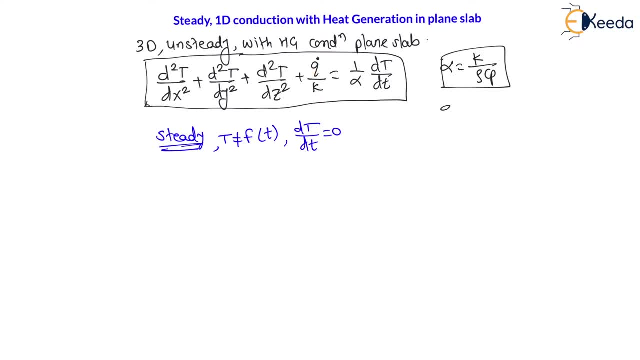 k is a thermal conductivity. q dot is a uniform heat generation rate. q dot is uniform heat generation rate, that is, heat generated per unit volume. That is heat generated per unit volume. This is called q dot And, my dear students, the unit is watt per meter cube for q dot. 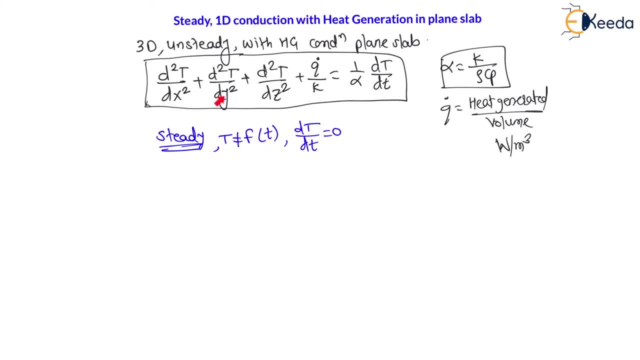 That k is a thermal conductivity in watt per meter kelvin, And x, y, z are directions. Now here, steady means the change in temperature with respect to time is zero. That is dt by dt. It means temperature is a function of only direction and one directional. 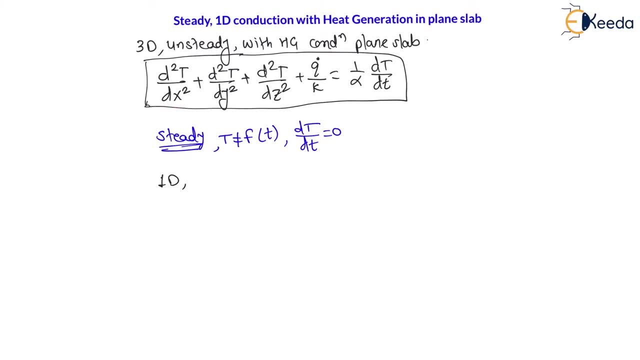 One directional means here. let us assume the heat transfer is along x direction. Therefore we can say, as we are assuming 1D, therefore d2t divided by dy square, which is equal to d2t, divided by dz square, will be equal to zero. 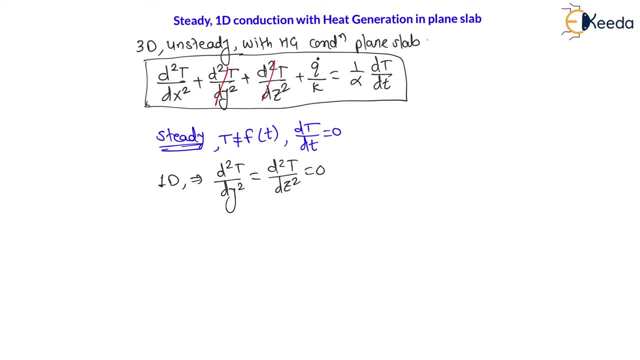 Therefore, my dear students, in this equation, as this term, this term and this term will be zero, therefore, the spatial condition that is steady, we can say steady, one directional, 1D, with heat generation, with heat generation in plane slab, in plane slab. 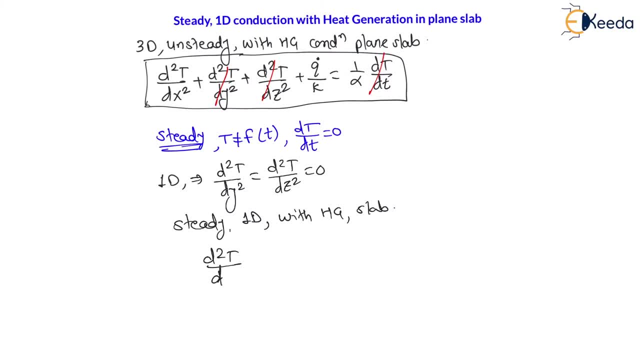 That equation will become: d2t divided by dx square plus q, dot by k is equal to zero. This will be the steady one directional with heat generation equation through the plane slab. Now let us do the analysis of this equation. My dear students, here the spatial case we got for one directional. 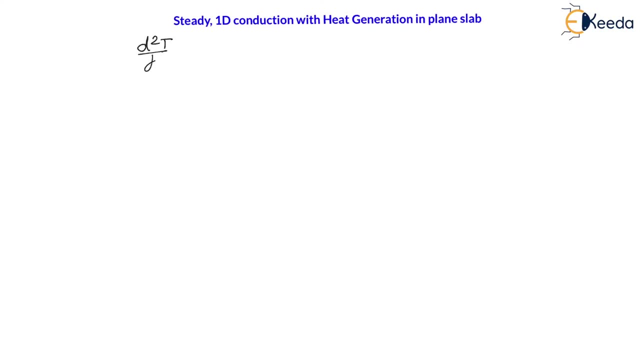 One directional steady state with heat generation. d2t divided by dx square plus q dot by k is equal to zero. This is the equation. Let us do the analysis of this equation Now. let us consider one plane slab. Let us say there is a plane slab like this: 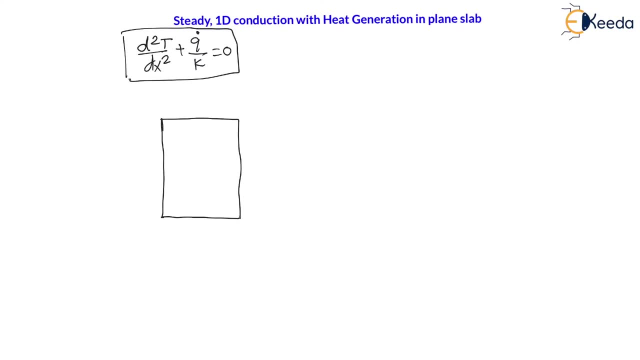 Here I am considering plane slab like this. Now, my dear students, in this slab, let us say the center line will be the x0. I am measuring the distance from center line. Let us say this is the center line Where distance x will be equal to zero. 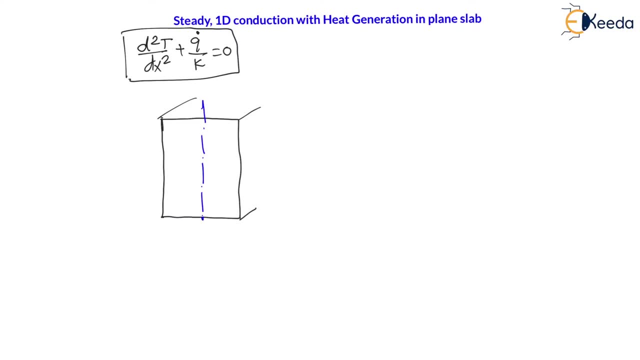 On this axis the distance x will be equal to zero, Means from the center we are going to measure the distance. Here x is equal to zero. And let us say the slab length is 2L. Here this distance is 2L. 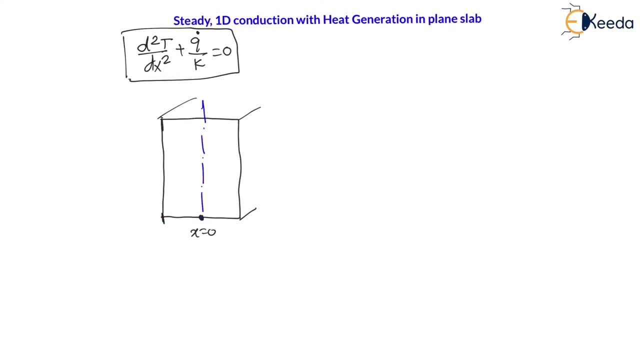 Therefore, here, at this location, as it is a left side, it will be minus L. Therefore, at this location, x will be equal to minus L And at this location, as this point is towards the right side, therefore, this location will be positive. 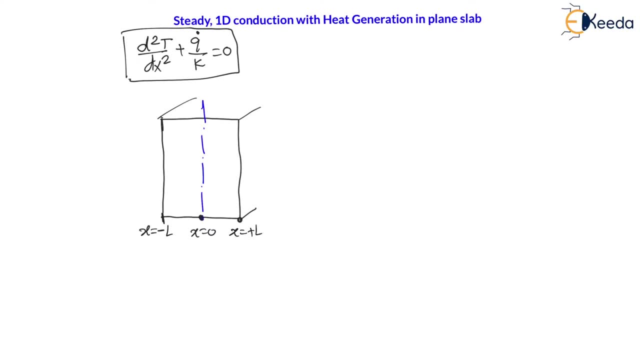 So I am considering right side, So I am considering right side, So I am considering left side. distance x is equal to plus l. this is our assumption, means the length of slab. this length of slab will be equal to 2n, that we are assuming right minus l to plus l right, and this is a 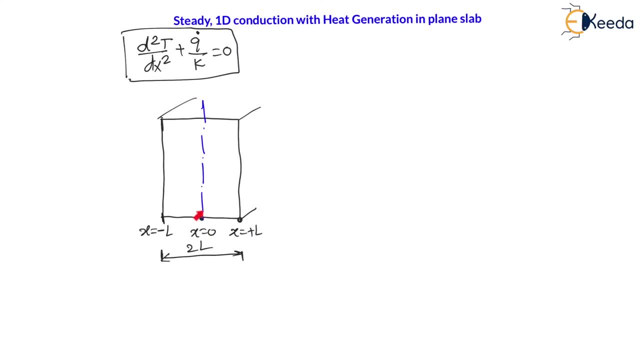 center line. now there is a significance for the center line. that's why i have considered this center line, now, my distance. let us consider here, as i have mentioned here, steady state. as we have mentioned here, steady state right means for steady state, whatever may be the heat. 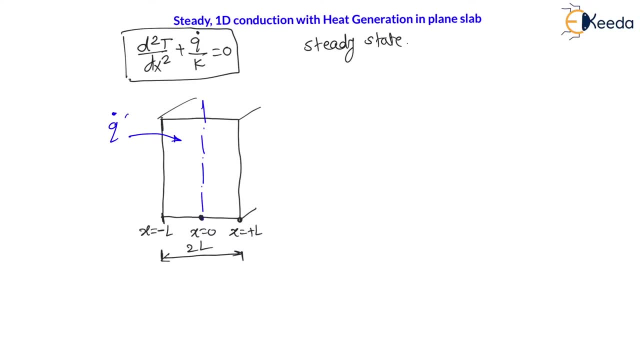 generated in the wall. the heat generated is q dot, which is nothing but heat generated per unit volume: watt per meter cube. now this heat generated in the slab must be equal to heat convected from the sides of wall right. therefore, whatever may be the heat generated, must be equal to heat. 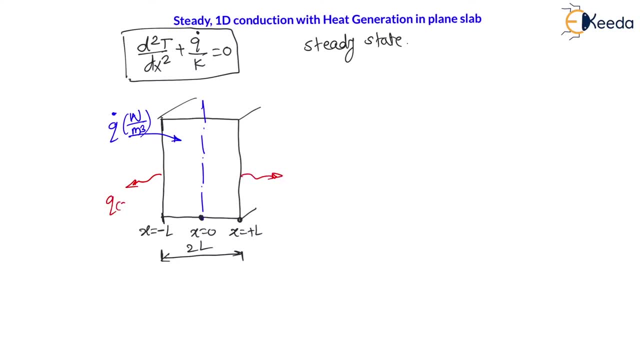 convected from both side of the slab right is equal to q convection. q convection from both side, there will be a convection heat transfer. right now, the meaning of steady state is nothing but temperature is not a function of time. that means the wall temperature at any instant of time remains constant. therefore, 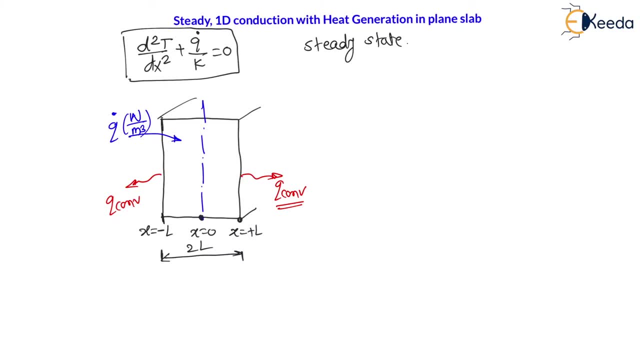 temperature of wall is always constant with respect to time. therefore, my dear students, to keep this wall temperature constant, whatever the heat generated within this plane slab must be equal to heat convected from the all surfaces. right, therefore, my dear students, for steady state condition, we can say: all the heat generated, all the heat generated must be equal to all the heat. 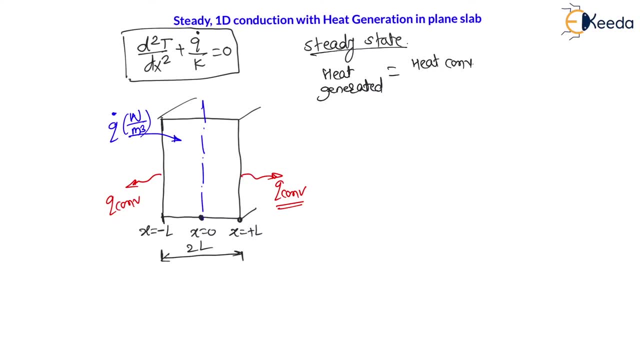 convected from all theody factor material, for all the heat generated earth material, which is all the heat convected right? so, my dear students, heat generated, which is nothing but q dot, is watt per meter cube. if i multiply this with volume, that is meter cube, then answer will be in watt. 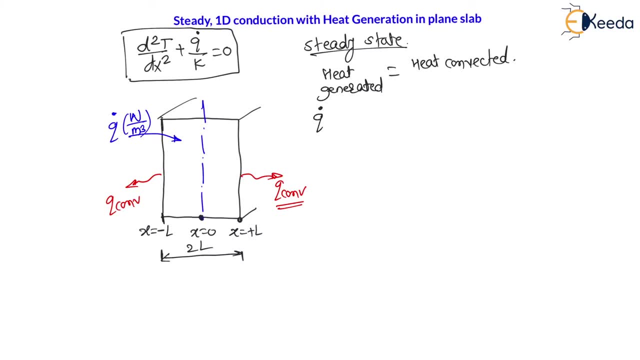 therefore, here heat generated is q dot, heat generation rate, q dot into volume, into volume, this is total heat generated is equal to total heat convected will be equal to h a. now here the temperature of wall. you want to consider temperature of wall and heat is convected from wall to surrounding, which is at temperature t, infinity. now the convection is: 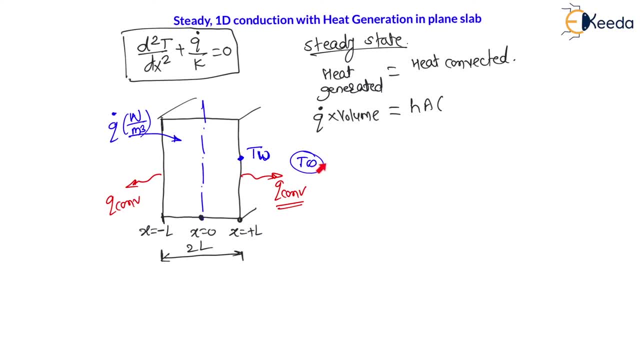 between wall and surrounding. surrounding, as is at temperature t infinity and wall is at temperature t wall. therefore, it will be equal to t wall minus t infinity. and right, and my dear students, here, a, this a is nothing but total exposed area. right, this a will be total contacting area or total exposed area between solid surface. 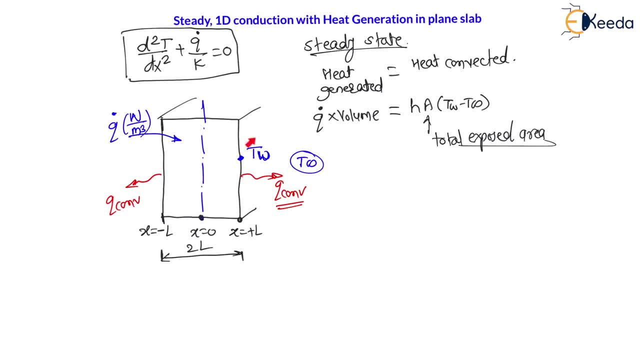 and the corresponding fluid right means if there is a convection from both side, then both area we have to consider. if convection is from all six side, then all six areas we have to consider over here and from this equation we will get the wall temperature right because we have fluid infinity. 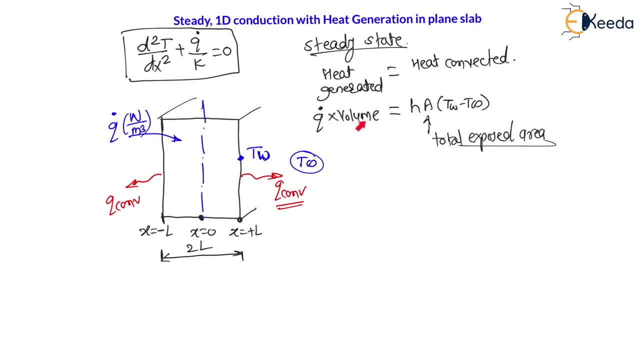 temperature, that is, fluid temperature, outside air temperature. we have volume, we can calculate q dot. they will provide in the examination, yes, they will provide area. you can calculate right, and from these you can calculate the wall temperature. now, my dear students, let us understand the analysis of this problem right now here. 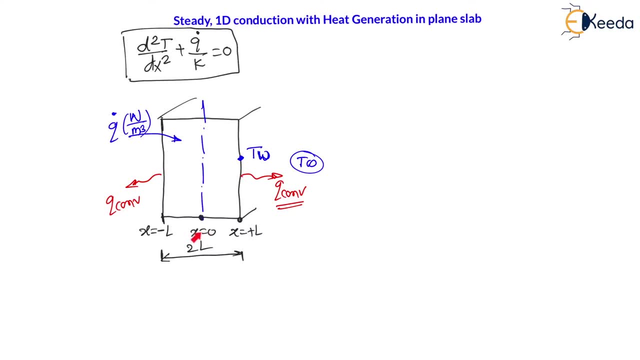 the. we are assuming the center line as x is equal to zero and here x is equal to minus l. x is equal to plus l means total length is 2l and by the equation of this equation we can find the temperature relationship. therefore, use the equation that is d2 t divided by dx square. 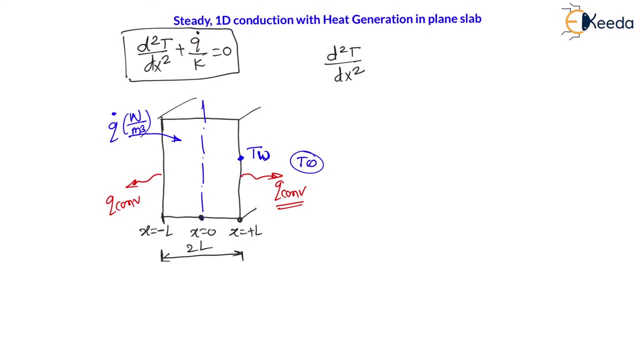 plus q dot by k is equal to zero. therefore, this q dot by k on this side, right side- it will become minus q dot by k. right. this is second derivative of temperature with respect to distance. so let us integrate this equation. if i integrate this equation, then i will get temperature gradient along x direction right. therefore, integration of d2 t divided by dx square will be equal to integration minus q dot by k. right, let us integrate right, without putting limits. if i integrate, there will be integration of d2 t divided by dx square will be equal to integration minus q dot by k. right, let us integrate right, without putting limits. if i integrate, there will be integration of d2 t divided by dx square will be equal to integration minus q dot by k. right, let us integrate right, without putting limits. if i integrate, there will be integration of d2 t divided by dx square will be equal to integration minus q dot by k. right, let us integrate right, without putting limits. if i integrate, there will be integration of d2 t divided by dx square will be equal to integration minus q dot by k. right, let us integrate right, without putting limits. if 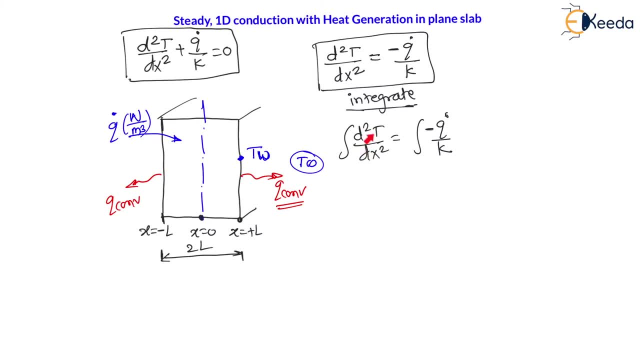 be an integration constant. therefore, my dear students, what is the integration of d2t divided by dx square? it is dt by dx will be equal to now. q, dot and k are constant. here this material will be having some thermal conductivity, k, and thermal conductivity k is constant as well as q dot is. 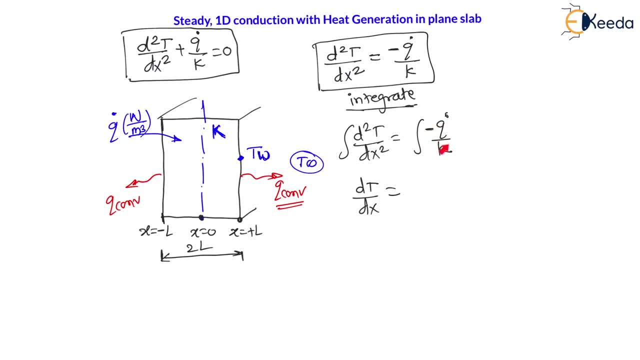 constant. in previous lecture all terminologies we have seen. so i have suggested at the start of lecture that watch my previous lecture, then come here right now, my dear students. therefore, minus q, dot by k will be constant, and here integration will be equal to x right plus. 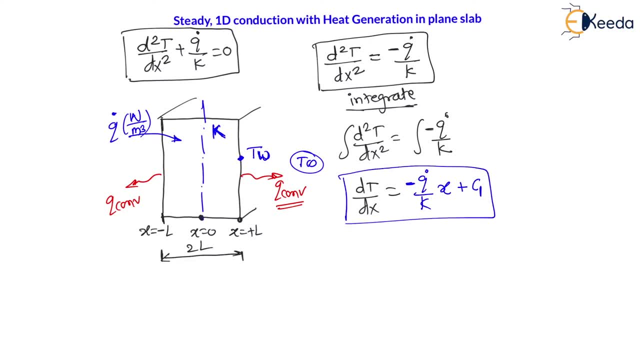 there will be an integration constant c1. as we have not kept the limits, there will be always integration constant. therefore, it will be minus q dot by k x, plus c1. right, this is called a temperature gradient equation. this is our first equation, which is temperature gradient equation. 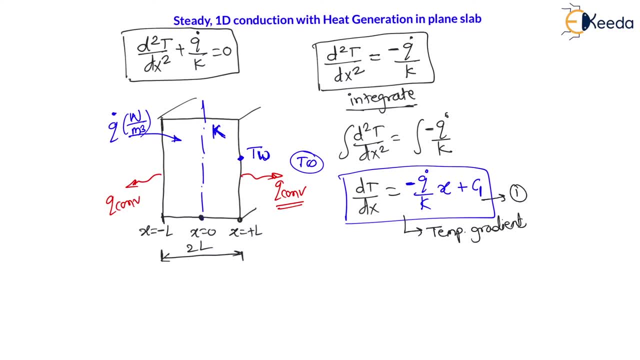 temperature gradient equation. right now, my dear students, again, let us you integrate this equation. again, integrate this equation. temperature graded equation. therefore, again, if i integrate this equation, i will get temperature profile. therefore, integration dt by dx will be equal to integration minus q, dot by kx plus t1. right, let us integrate this equation. 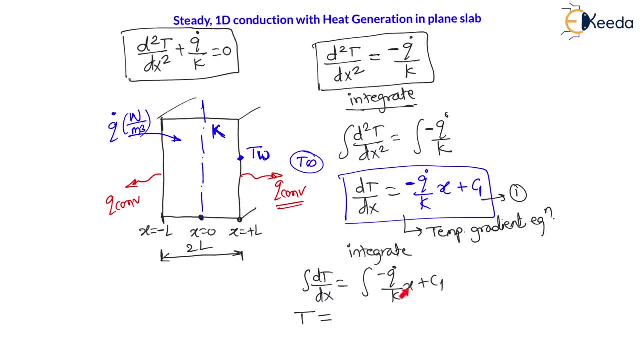 therefore i will get: temperature is equal to now, integration of x will be x square by 2. therefore, here, minus q dot x square, minus q dot x square divided by 2k, plus integration of constant will be constant into x plus there will be new integration constant, c2, right again after. 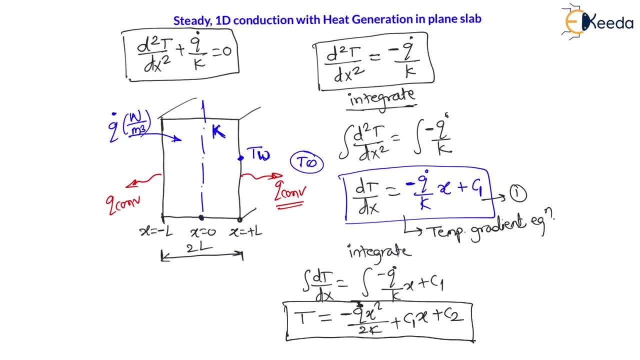 every integration, there is always integration constant right. therefore, there will be a new integration of c2. this is the second equation and this equation is temperature profile. temperature equation right or temperature profile. temperature distribution will be calculated with help of this equation and, my dear students here, c1 and c2 are the integration constants during first integration. 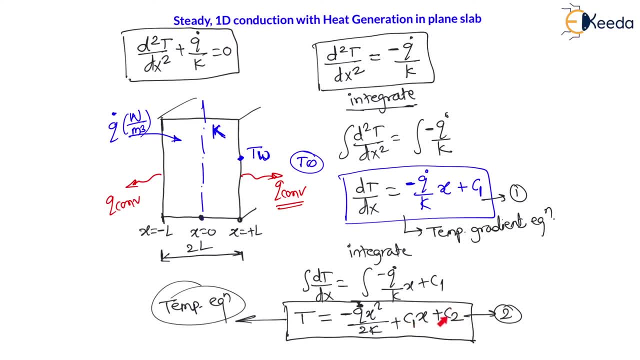 c1 is a constant. during second integration, c2 is a constant. and these constants we have to calculate with the help of boundary conditions, right? so let us understand these boundary conditions. there are various types of special cases, such like both walls are at subjected to different temperature. both walls subject to different temperature, then whatever may be the 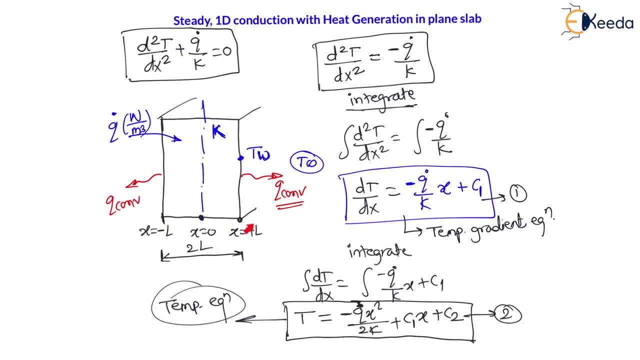 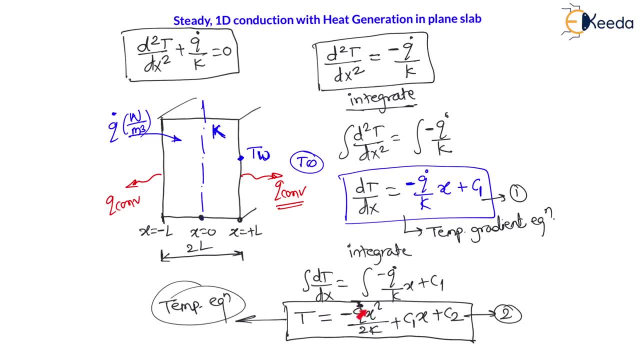 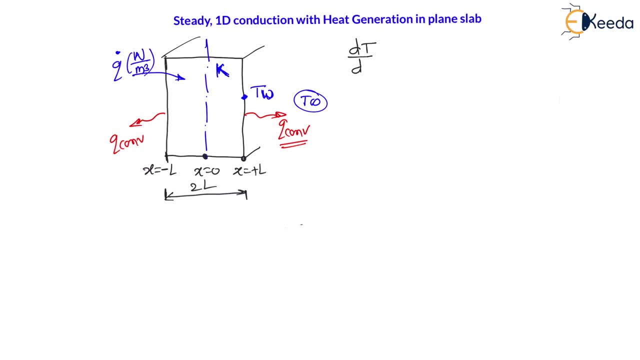 to distance, then at this particular x is equal to distance, then at this particular x is equal. use this temperature gradient equation and temperature equation. let us write down them and look at the special cases. so the first equation, that is temperature gradient equation, is: dt by dx is equal to minus q. dot by k into x plus c1. this is our first equation of temperature. 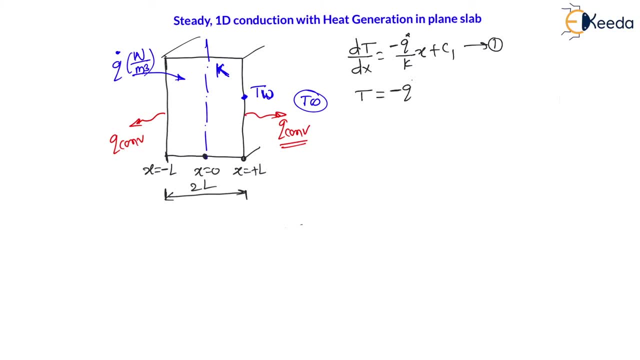 gradient. and second equation is temperature profile, which is minus q dot x squared divided by 2k plus c1, x plus c2. this is our second equation, that is, temperature profile equation. right now, my dear students, let us observe the special cases here we are going to understand. 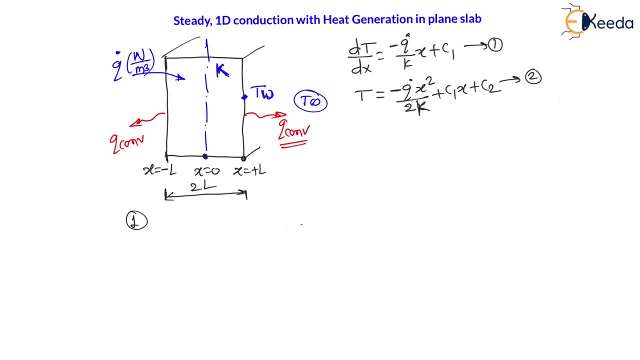 first special case, very first special case, is if both sides of slab are maintained at same temperature, if both sides of slab at same wall temperature, same wall temperature. right, that means on left side there will be a wall temperature p wall, and as well as on right side there will be a wall temperature p wall. so let us consider here on left: 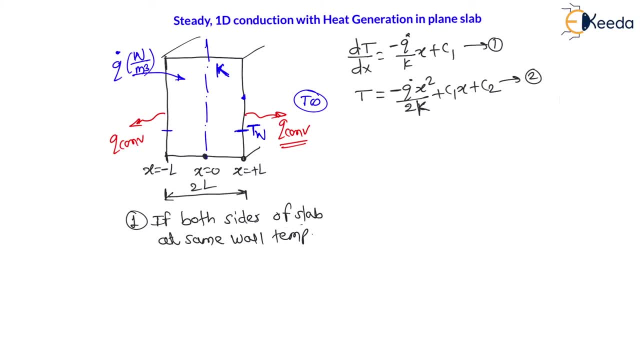 right side wall temperature is p wall, as well as on right side the wall temperature is p wall, which are same, the constant temperature on both sides. right now, for this case, let us find the temperature profile and temperature distribution here, right now, my dear students, therefore, the boundary condition, here we can say the boundary conditions are very first boundary condition, right. 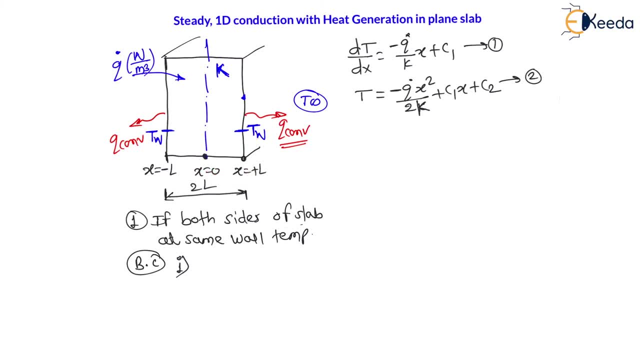 x is equal to plus, here temperature will be equal to t wall. therefore, x is equal to plus l, temperature is equal to t one. this is the first boundary condition. second boundary condition is: whenever x is equal to minus l right this left side, then temperature is equal to t wall temperature is. 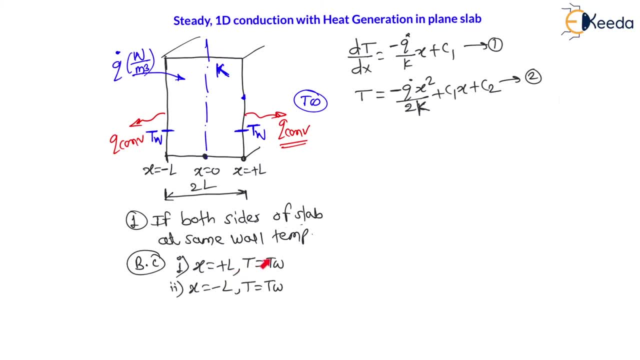 equal to p wall, right? with the help of these two boundary conditions we will get in one of the integration constant. so let us put these two boundary conditions in equation number two, right? so if i use equation number two and substitute boundary conditions, then my dear students put the 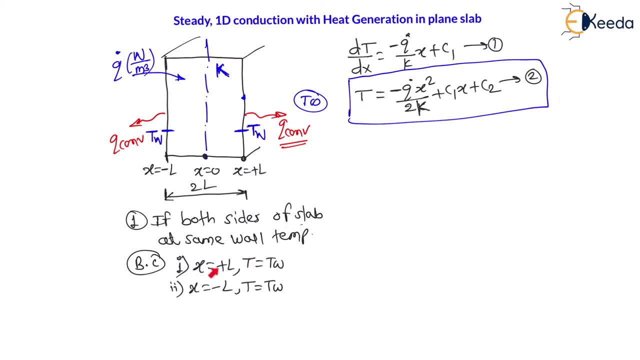 first boundary condition. therefore, if i put here temperature equal to p wall and x is equal to l, let us derive this equation. therefore, p wall will be equal to minus q. x is l square divided by 2k plus c1 l. x is l plus c2. right again, if i use second boundary condition, that is, x is equal to minus l t. 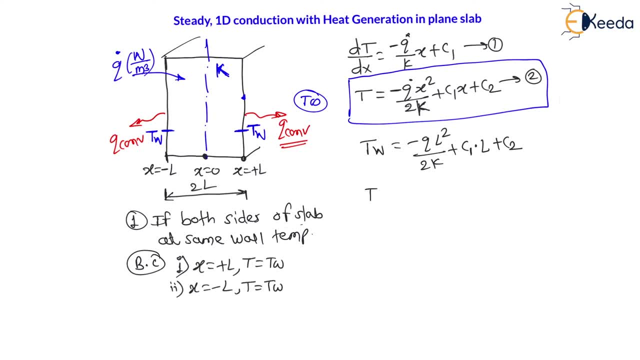 is equal to p wall. let us put here: temperature is p wall, x is minus l. therefore minus l square will be equal to l square, only therefore minus q dot. here it is a q dot l square divided by 2k plus. now here c1 into minus l minus. 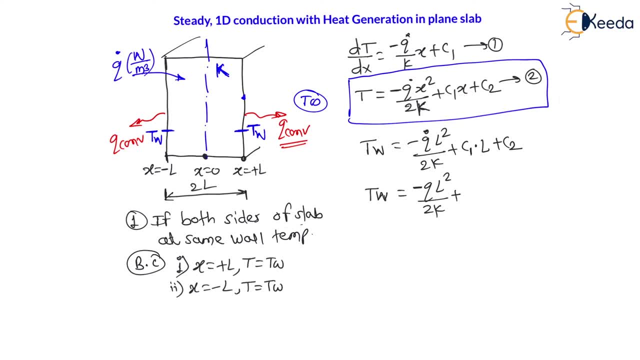 c1 l. right, it will become minus c1 l. therefore, here, instead of plus sign, there will be a minus sign. therefore, the equation will become minus c1 l, plus c2, right, my dear students, let us subtract these two equations. if i subtract equation number two from the equation number one, 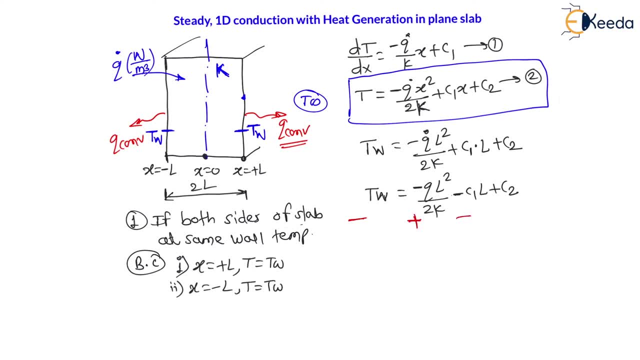 here minus, this minus minus will become plus, here minus will become plus and this plus will become minus. if i subtract these equations right, then this p wall t wall get cancelled here. this p wall t wall get cancelled. this minus and plus term get cancelled. plus c2 minus c2 will get cancelled. 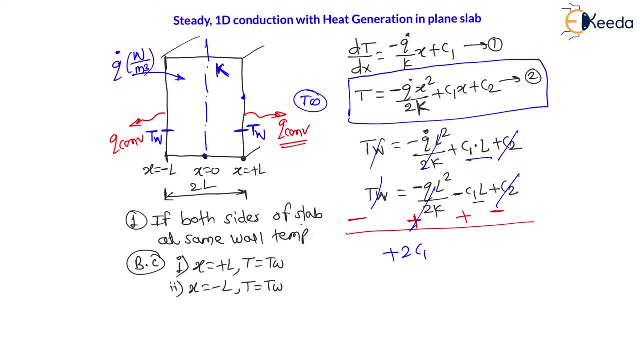 and this will be plus. plus means plus twice. c1- l will be equal to zero. Right And length is not 0. That means the first integration constant, C1, must be equal to 0.. So, my dear students, here we have calculated first integration constant. 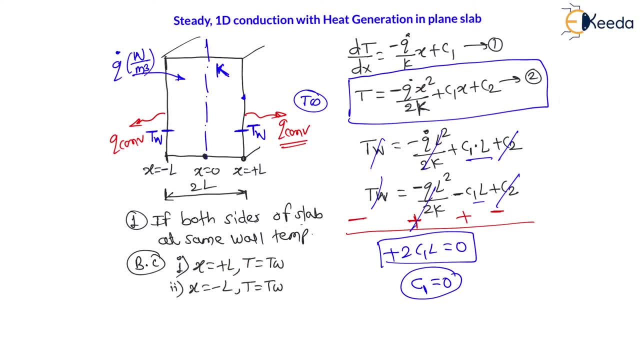 Let us modify these equations again From the first boundary condition we have got, first integration constant, that is, C1 is equal to 0. Let us put here in temperature profile temperature gradient and temperature profile, Right? So, my dear students, let us put these equations. 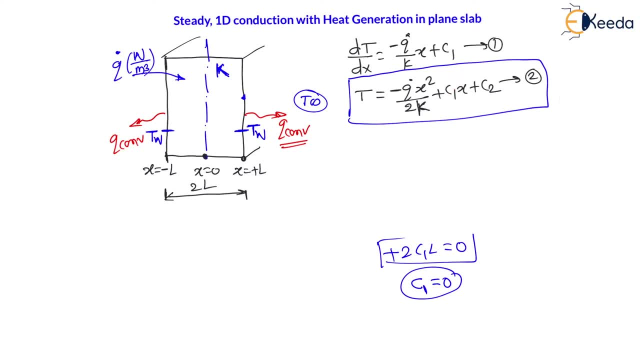 So in these equations, if I put C1 is equal to 0, then here this C1 term will go Right. This will be the first equation. This C1 term will go. This will be the second equation. Therefore, the modified equation becomes: 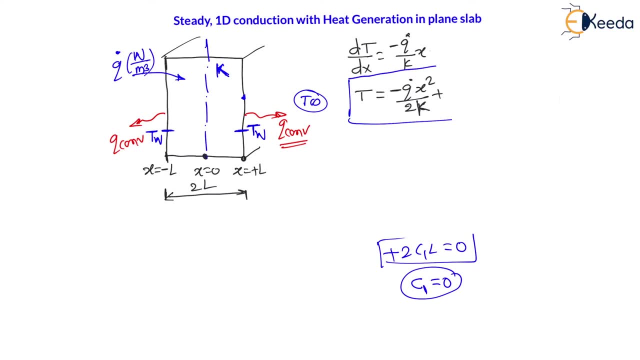 Right. Here. the modified equation becomes Right After calculation of C1.. DT by DX will be equal to Q dot by K into X. This is the first equation And temperature is equal to minus Q dot X square divided by 2K plus Q2.. 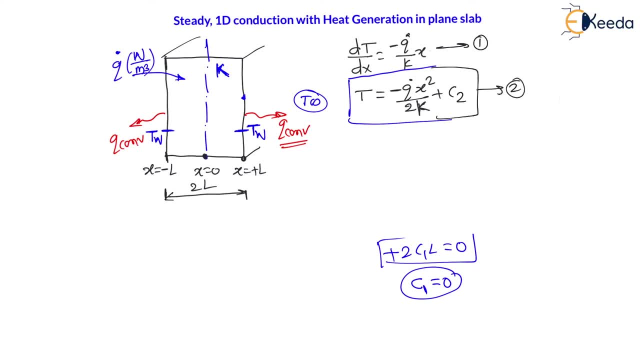 This will be our second equation. This will be our second equation. Right, These are the modified equations. after putting, C1 is equal to 0.. Right Now, my dear students, we know that for temperature to be maximum, second boundary condition, 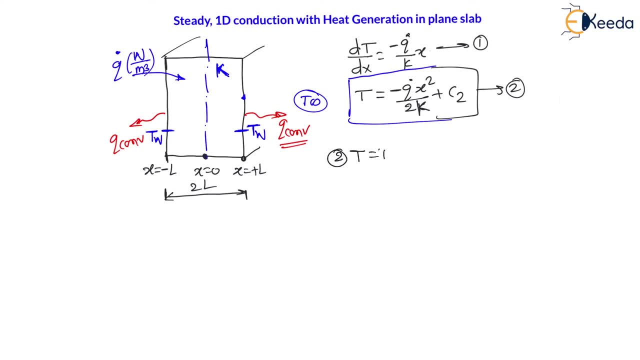 Here we are getting second boundary condition, That is, for temperature to be maximum. As, per mathematics, this change in temperature with respect to distance must be equal to 0.. That is, temperature gradient along X direction must be equal to 0.. Therefore, here equate, this temperature gradient is equal to 0.. 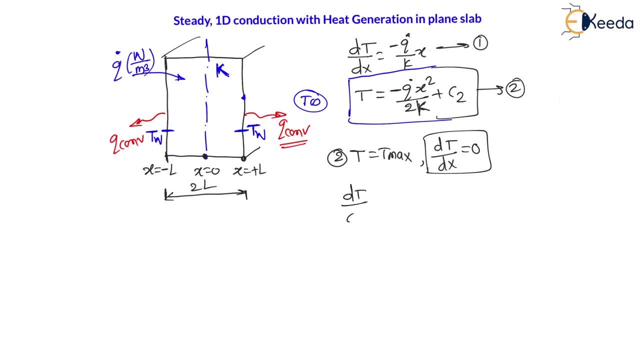 Therefore, for temperature to be maximum, DT by DX, which is equal to minus Q, dot by KX must be equal to 0.. Now Q? dot is uniform heat generation rate, K is thermal conductivity. These two values are not 0.. 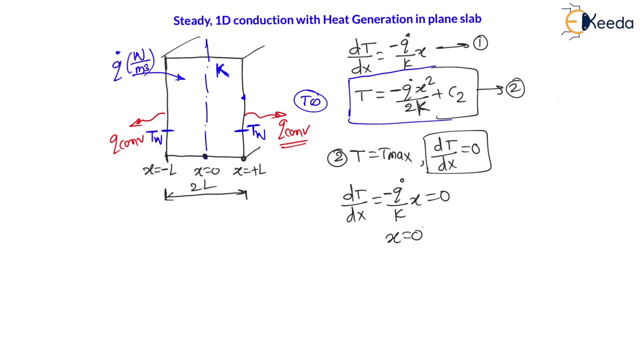 Therefore, here X must be 0. From this we will get: X is equal to 0. Means, my dear students, whenever X is 0, then temperature will be equal to maximum temperature. Temperature will be equal to maximum temperature. 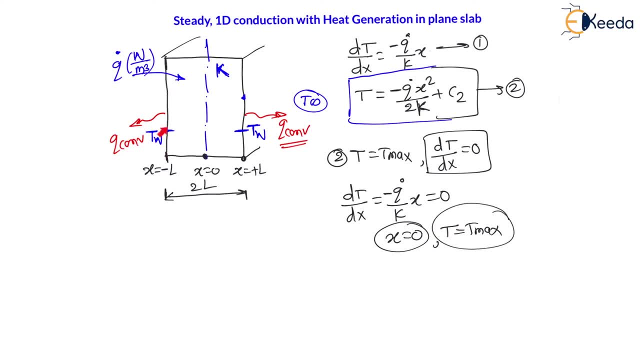 This will be our second boundary condition. Right, Whenever X is equal to minus CL or X is equal to plus CL, Temperature is equal to T wall, And whenever X is equal to 0, temperature will be maximum temperature. This will be our second boundary condition. 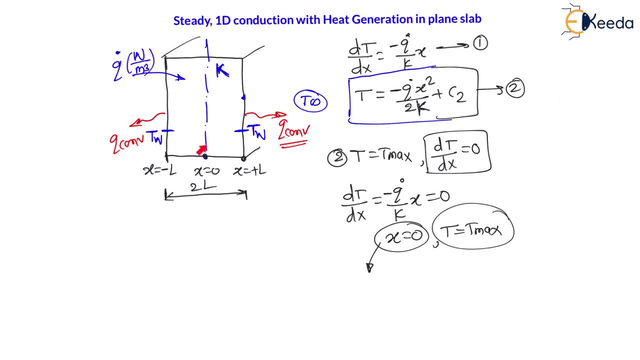 That means, my dear students, X is equal to 0 is the center line. Therefore, for the special case having both sides of wall at same temperature, the maximum temperature will be at center. Therefore, if wall temperature is same for both sides, the maximum temperature will be at center. 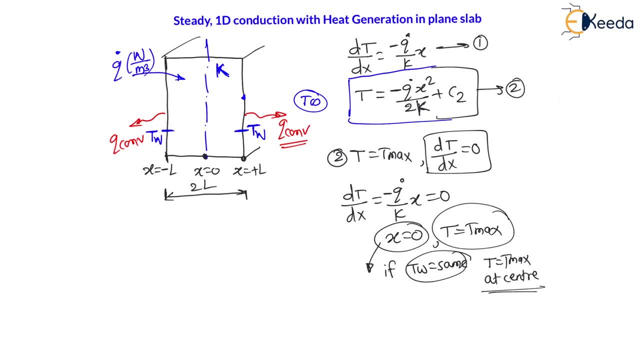 At center line. Right. This is very important. Straight forward in examination they will ask question on this statement also Right. So mark here maximum temperature point. Therefore, if I mark here maximum temperature point, let us say at this point, center line, the temperature is maximum. 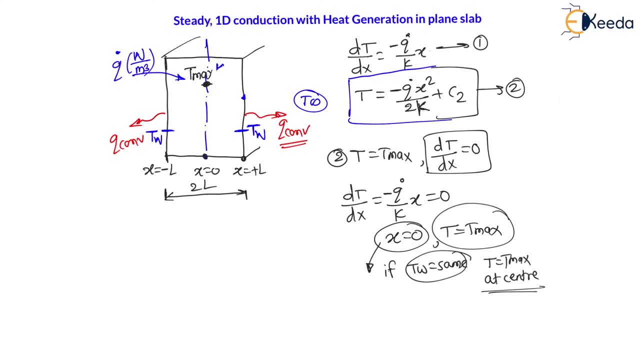 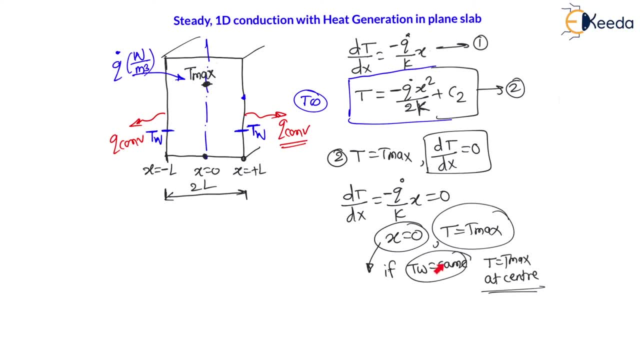 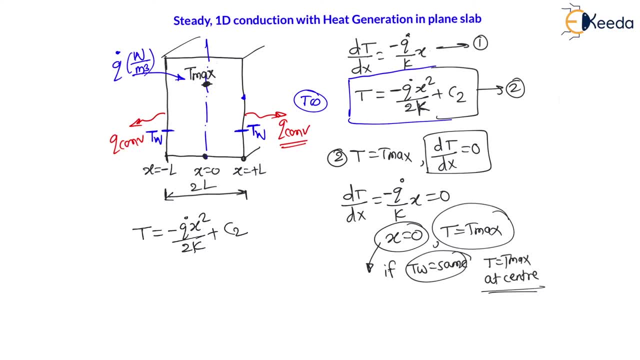 C2.. Now let us substitute this condition, That is, X is equal to 0,, temperature will be maximum, Right? Therefore we will get: maximum temperature is equal to. if I put, X is equal to 0, is equal to C2.. 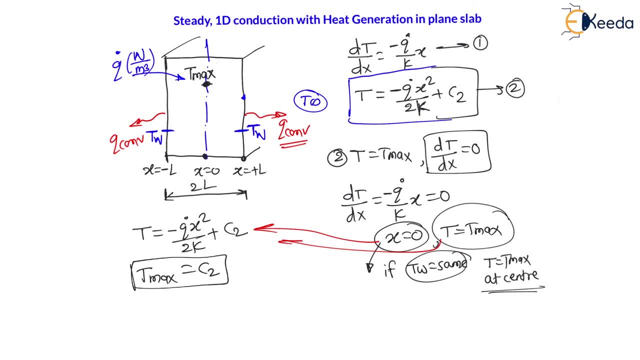 Therefore, my dear students, let us put this condition. dear students, from this condition we are getting another boundary condition. firstly, we have calculated boundary condition: c1 is equal to 0. now c2 is equal to maximum temperature. so let us use this c2 in this equation, equation number two, right temperature profile equation. from this we will get: 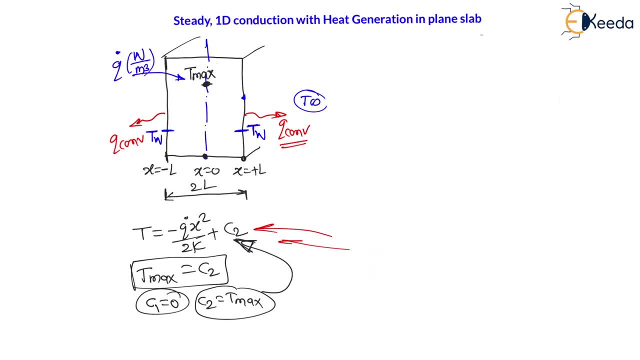 temperature profile, right, so let us write down this temperature profile, final temperature profile, right? therefore, my dear students, this temperature profile, which is nothing but temperature, is equal to minus q, dot x square divided by 2k plus c2, right, and this c2 is nothing but maximum. 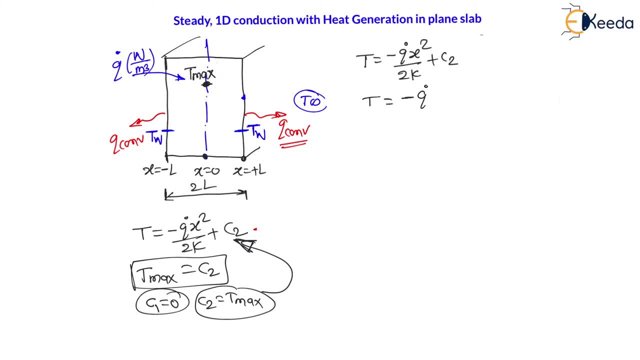 temperature. therefore, temperature is equal to minus q dot x square divided by 2k, plus maximum temperature. from this we will get maximum temperature in the cycle. minus temperature will be equal to here. it will become plus q dot x square divided by 2k. right, this will be the. 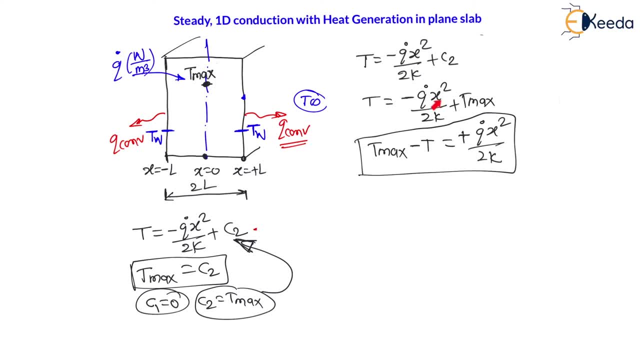 temperature profile. so, my dear students, can i say this: temperature is directly proportional to x square. right, as temperature is directly proportional to x square, and as it is negative, means as x increases, temperature decreases. likewise, whenever x is equal to 0, temperature is maximum, and as it is negative, x increases. on both sides, temperature decreases on. 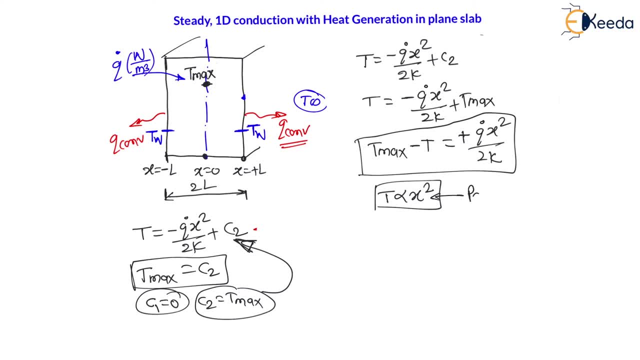 both sides. right, therefore, the distribution, temperature distribution will be parabolic. the temperature distribution will be parabolic. right. and, my dear students, we have one more boundary condition, that is, whenever x is equal to plus l or whenever x is equal to minus l. right means both x remains, both x remains. temperature is wall temperature. 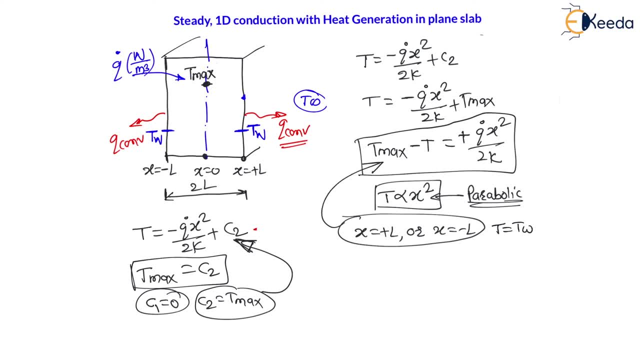 temperature will be equal to wall temperature. so let us put this boundary condition in the equation. therefore, maximum temperature minus wall temperature will be equal to plus q, dot x square divided by 2k. right, this will be the equation and my dear students in examination, directly straight forward, they will ask you question: what is the maximum temperature minus wall? 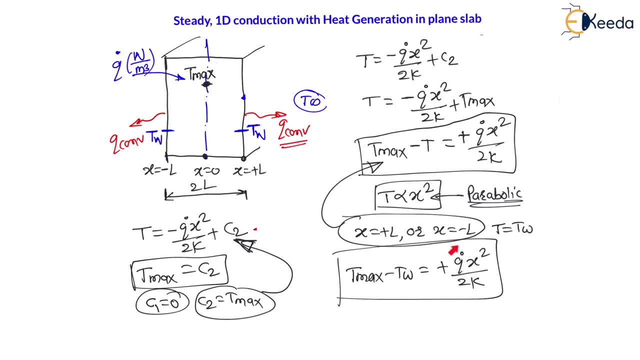 temperature. it is q dot x squared over 2 k. here, instead of x, we have to put l. therefore, if i put minus l or plus l, it will become l square, only right. therefore, replace this x square with el square right, replace x square with l square. therefore the equation becomes q dot el squared. 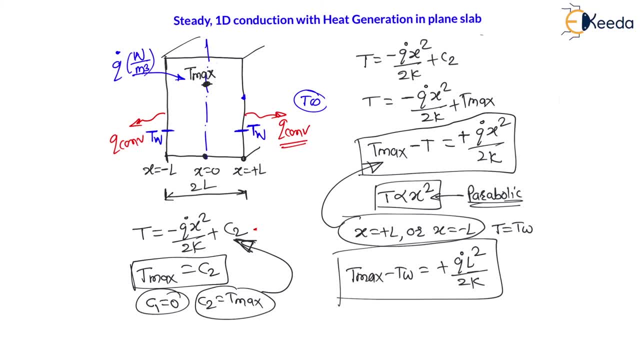 by 2k. now, maximum temperature is on the center line. therefore, many times in the examination they will ask you what is the difference of center engine temperature and wall temperature? it is 2.1 L temperature minus wall temperature. it is q dot L squared divided by 2k. and, my dear students, how to? 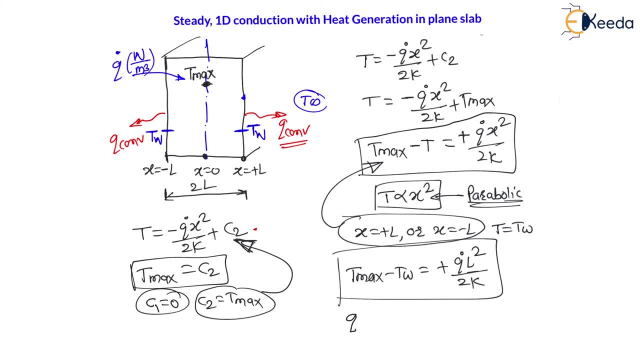 find this wall temperature right. whatever may be heat generated. that is, q dot into volume. is heat generated must be equal to heat convicted from the both side, right that is it converted. is h a p wall minus t, infinity, right that already we have seen this. from this equation we will find: 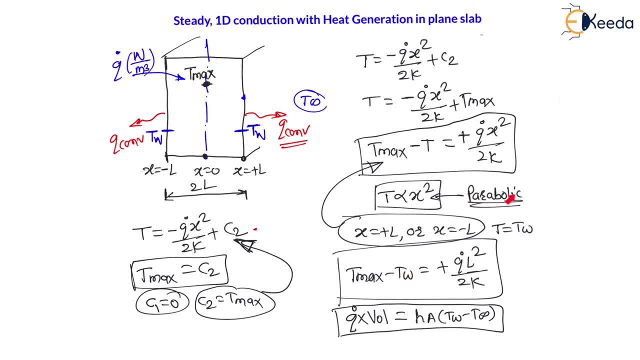 wall temperature to substitute it here. right, and the distribution will be parabolic. right, and my dear students, the maximum temperature will be on center line and from here the heat flow is always from maximum temperature to minimum temperature. therefore, the distribution will be parabolic, that is, it will flow from maximum temperature to wall temperature parabolically. right, it will flow from. 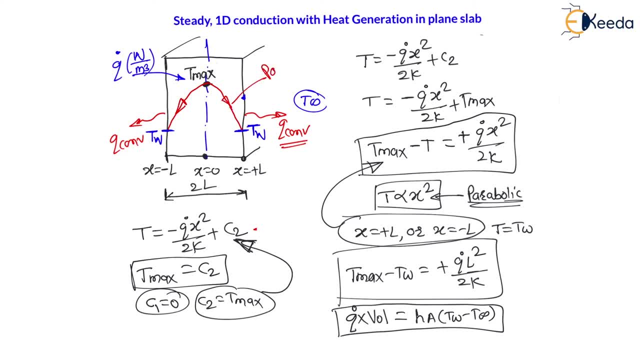 maximum temperature to wall temperature parabolically, and this graph will be parabolic. this temperature distribution will be parabolic and the heat transfer will be from center to wall, center to wall, on both sides. this will be the direction of heat transfer. many times in examination they will ask you what is the? 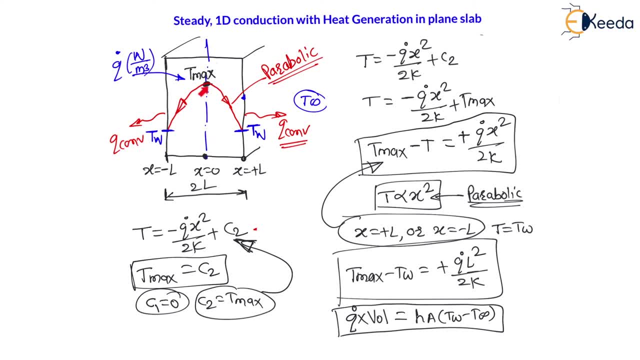 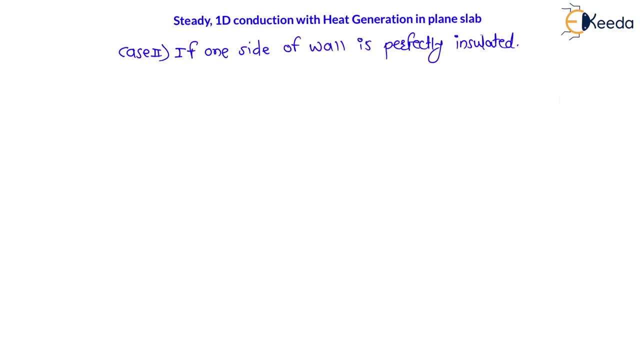 direction of heat transfer. also, therefore, the direction of heat transfer will be from center to wall, from center to wall, that is, from maximum temperature to minimum temperature. now, first special case we have seen: both sides of wall are subjected to same temperature. now, second special case, we will see: if one side of wall is perfectly insulated, then what will be the location of? 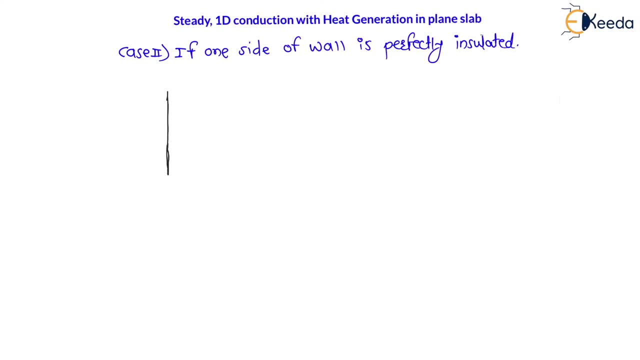 maximum temperature right now. if both sides are subjected to same temperature, then the location of maximum temperature was center point. now here, if one side is insulated, this let us say: this side is insulated, it is insulated end left side, i am assuming. insulated right now. for such cases, what? 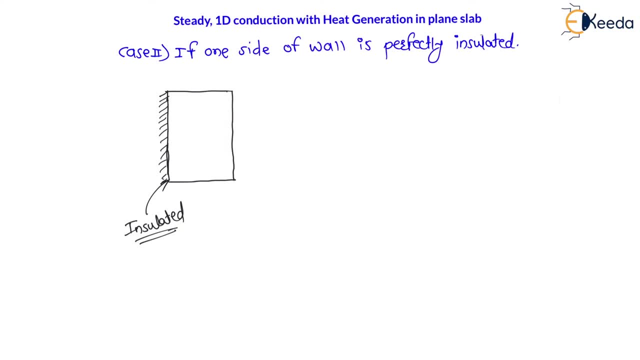 will be the location of maximum temperature and what will be the temperature profile. the temperature profile is definitely parabolic. that already we have seen. now, location of maximum temperature, we are going to understand you. between: the heat conducted from insulated end will be equal to zero. heat conducted from the insulated end will be equal to zero, as well as heat convicted from 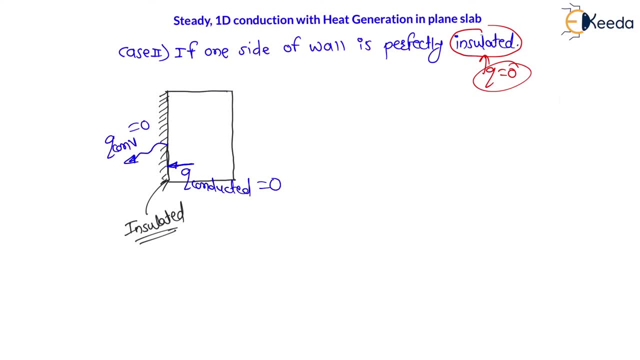 the insulated end will be also zero. heat convicted from the insulated end will be zero. any kind of heat transfer will be zero. therefore, as we can say, q conducted conduction heat transfer through insulated end to insulated end will be equal to zero and conduction heat transfer is nothing but. 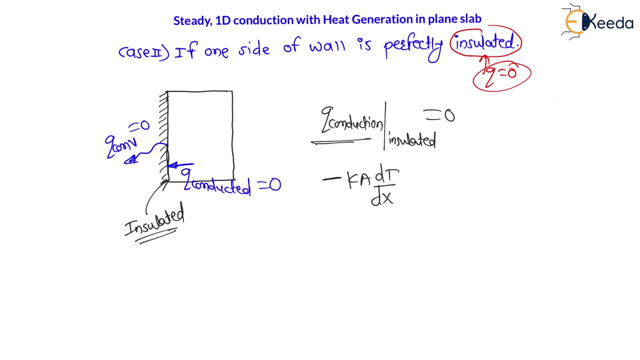 minus k a dt by dx, minus k a dt by dx through insulated end to insulated end is equal zero. now, thermal conductivity is not zero. this material is having some thermal conductivity k, again at insulated end. there is some area right. there will be some area, this area right, here, this. 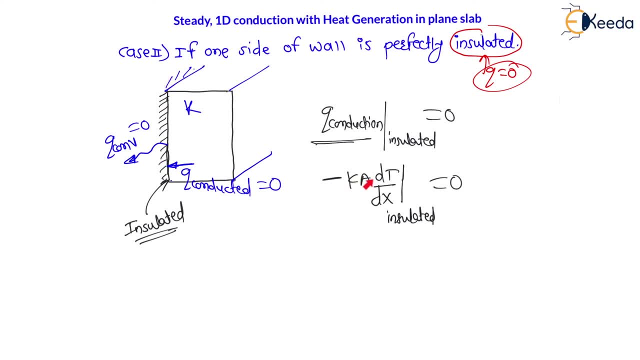 z dimension into y dimension. therefore, area is not zero, k is not zero. therefore, at insulated end, dt by dx- dt by dx- must be equal to zero. at insulated end must be equal to zero. that means the temperature change with respect to distance is zero. that means the temperature is maximum. 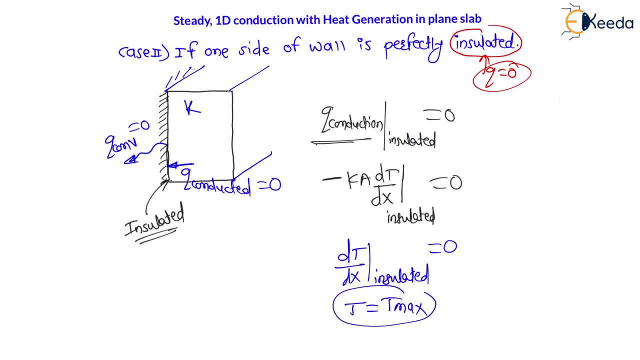 this is the condition for maximum temperature or not? therefore, the maximum temperature will be at insulated end, right. if one of the end is insulated, the maximum temperature will be at insulated end, right. therefore, here we got the maximum temperature point. the maximum temperature point is at insulated end, so mark this point. therefore, at this location, the temperature will